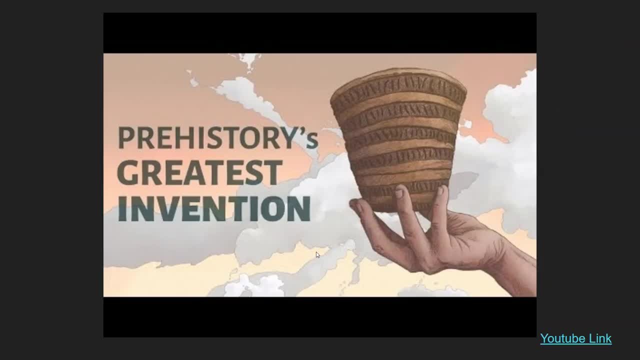 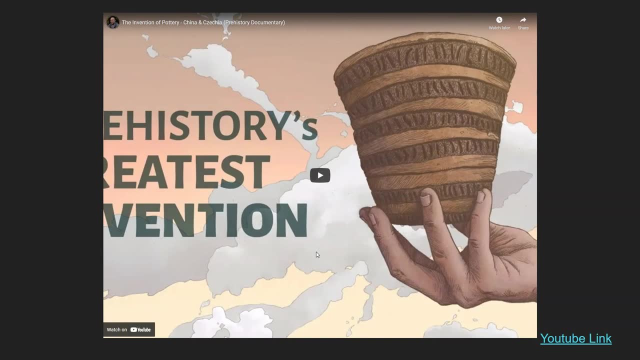 common nowadays. Anyways, let's get a little bit deeper into things. Also, I'll be linking this video in the description below, because it is a really cool sort of- like you know- explanation of, like, the history of pottery. okay, Pottery has been around. 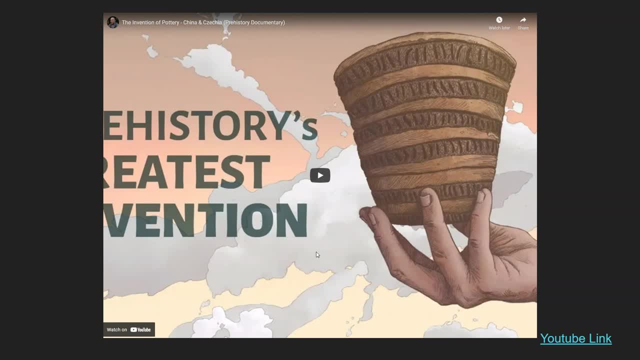 since the Neolithic, prehistoric kind of times and talks about where it kind of came from and all that kind of stuff. So definitely check out this video if you have a chance. Anyways, moving on, So we have clay, and clay is defined as a natural material, Natural meaning it comes from. 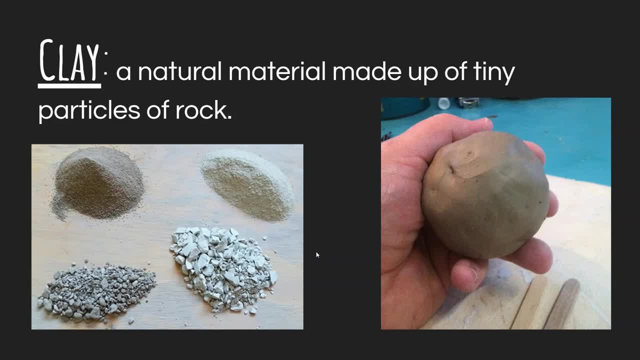 the earth. okay, We don't, as men, make clay. We take materials and you know, you know create clay with what's already here, so it's not made in a lab or nothing like that, And basically it's tiny particles of. 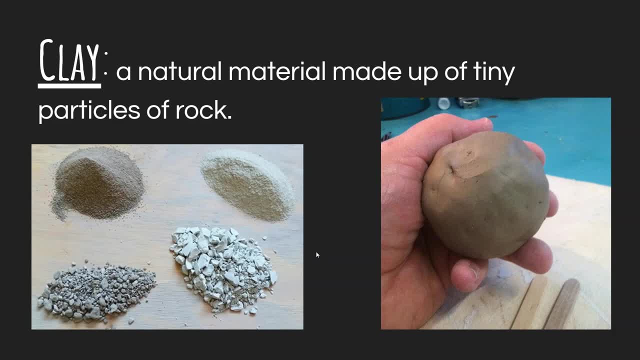 rock. okay, You take a rock, you smash it down, really good. add some water, boom, you got clay. okay, So that stuff over here turns into the nice workable clay that we end up using in class to make ceramic pieces, all right. And when we work with clay, 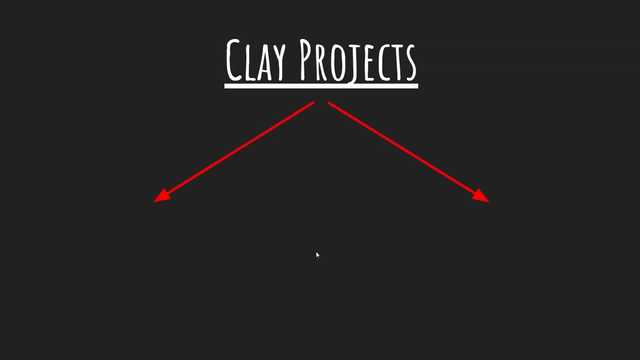 and make clay projects. we have two big categories that we're actually kind of working with. okay, There's wheel throwing clay and there's also hand building clay. Then there's a couple other different types, depending on how you're working with the clay and things. 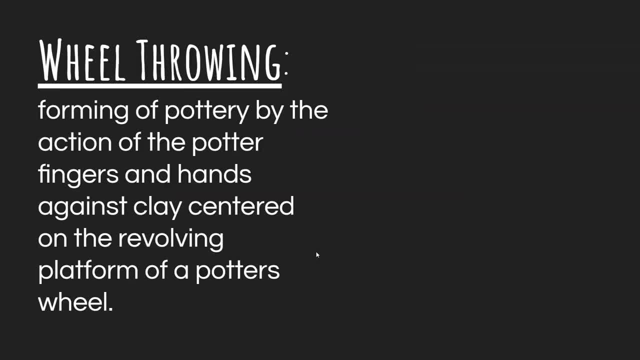 like that. Wheel throwing is forming the pottery by the action of the potter's fingers and hands against the clay centered on a revolving platform of a potter's wheel. Basically, that's a long way to describe what this guy's doing here. okay, Got a big hunk of clay. 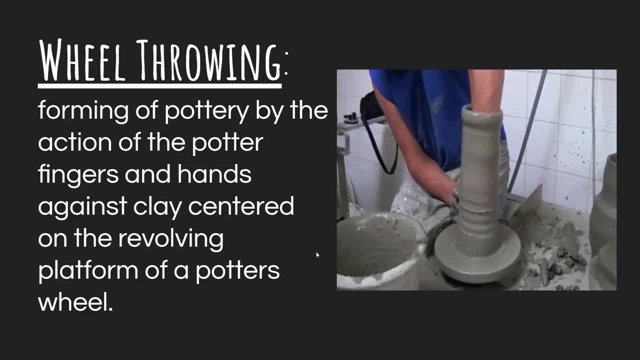 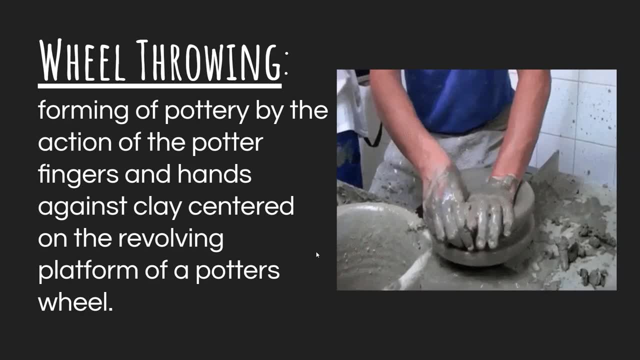 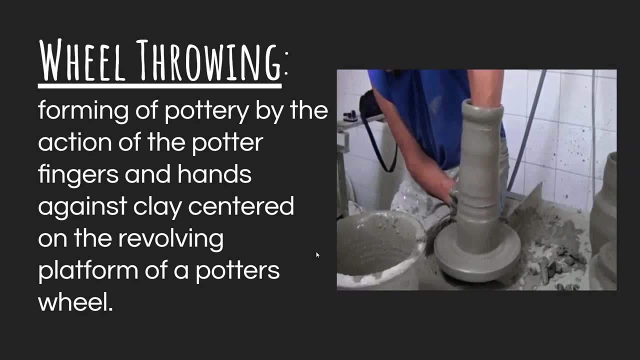 macking on this wheel that goes spinny, spinny, spinny And, based on pulling the clay and raising the clay up, you're actually able to form a pot, which is like crazy awesome, And it is a lot harder than it looks until you get used to it, And then you can start, you know, whipping out, you know. 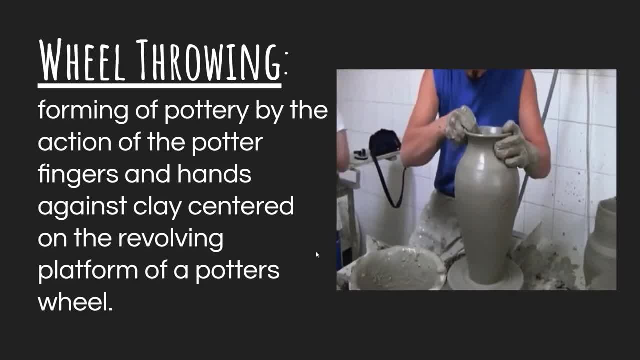 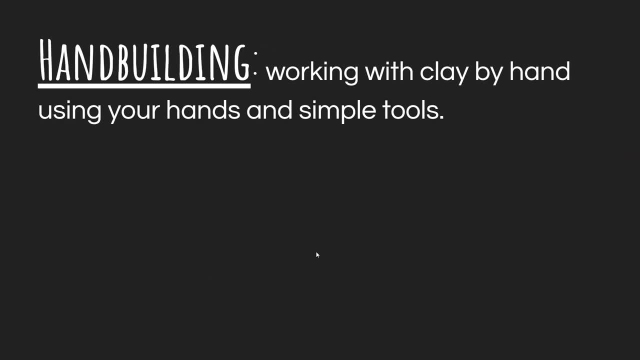 30, 40 cups a day, basically, But anyways, super fun. If you ever have a chance, definitely try wheel throwing. The other kind of category we talk about is something called hand building, And that's working with the clay, with your hands, obviously, and using simple tools in addition to 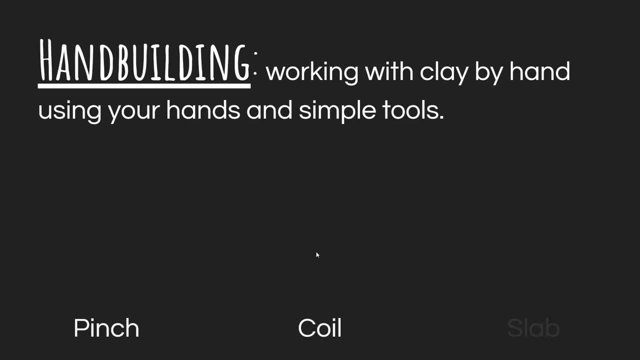 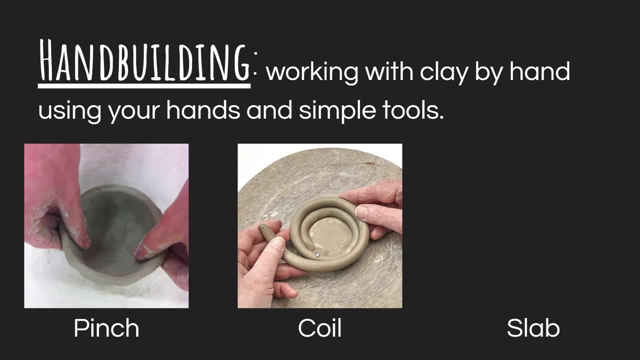 your hands to create it. And there's three big categories: We got pinch, we got coil and we got slab. okay, And they are very fancy named. okay, Pinch is, you know, when you pinch the clay to influence where it goes. And then, with coil, you roll out these long, skinny coils and stick them. 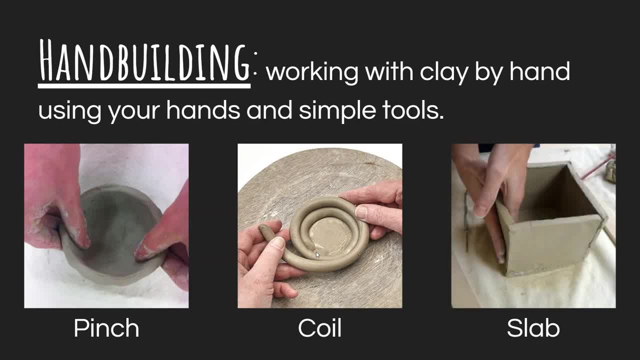 together And then you got slab, where you're rolling out flat slabs of clay and then sticking okay. So those are the big different categories that you can use to work with. you know your clay And you don't have to just do pinch or just coil, just slab. A lot of artists mix and match these. 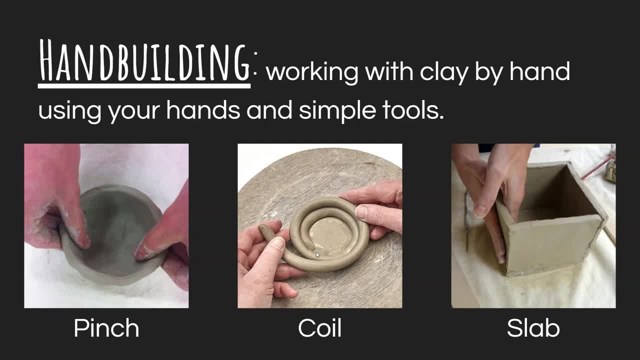 things depending on what they want with their clay piece. okay, So some techniques work better for other things, such as if I was trying to make something that's more like a cube. if I'm trying to make like a clay Rubik's cube or something like that, I probably want to use slab okay. 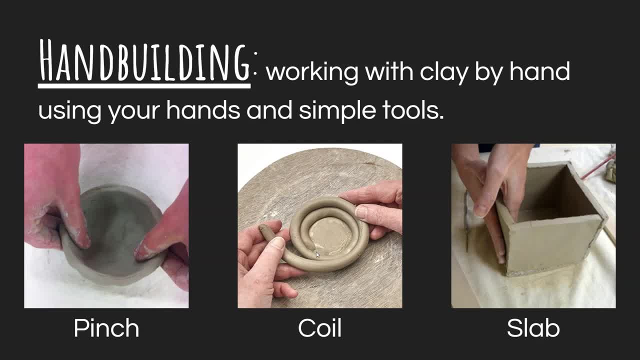 And if I'm trying to make something that's more like a cube, I probably want to use slab, okay, And if I'm trying to do something wrong- not something wrong, something round, like if I was trying to like make I don't know- a beam bag, I don't know, I'm trying to think of something. 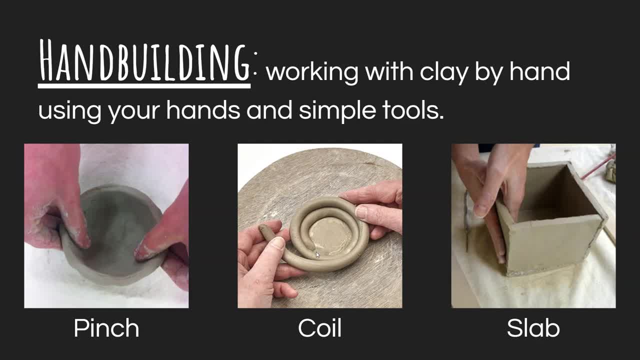 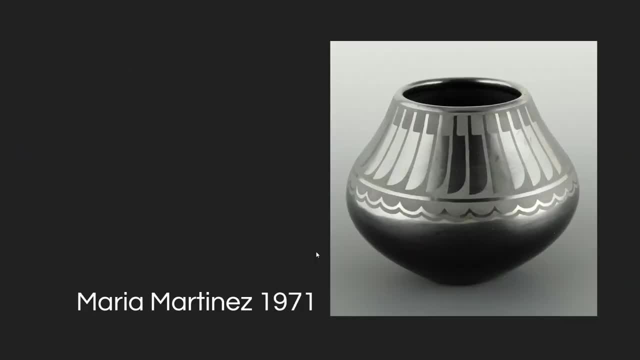 round or squishy, you know, Maybe slab's not the best choice and maybe pinch would work better, or maybe coil could help me, you know, get the curves just right, I don't know. Anyways, so there's a couple artists I really want to talk about. that are some. some of them are really big influencers. 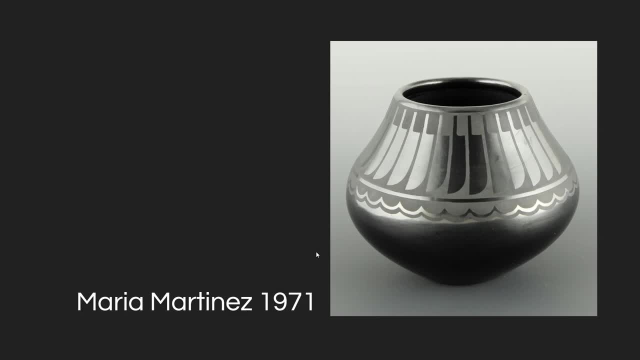 in ceramics and some of them are just really cool. They have really unique stuff. And the first is Maria Martinez, And she and her husband sort of created this black on black pottery style And they lived in the San Ildefonso Pueblo. Okay, I'll link the name in below. I probably can't even say 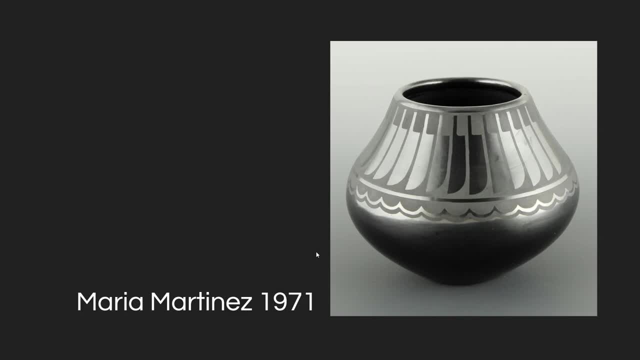 it right, But they lived in the Pueblo and they made their own clay. They went up the mountains, they grounded up the stone, they add water. So they made from start to finish each piece by hand, which is so cool. Through trial and error, they played around with different ways of creating these pieces and finish. 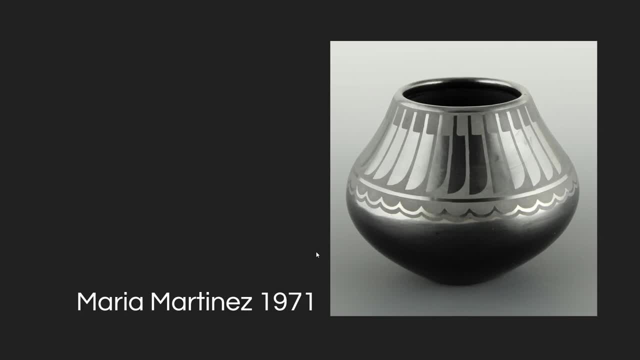 these pieces and ended up with something very unique. Okay, They used a lot of coil in building the bodies of their clay pieces And they also burnished it, which is how we describe like they polished it. they had like a special stone And when they rubbed it on the surface of the clay, 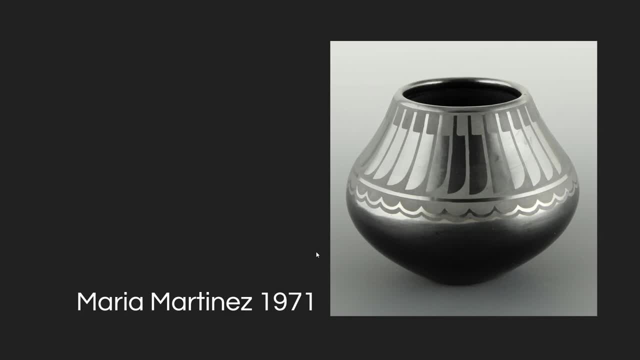 got it like super, super smooth and shiny, And then they would paint this iron oxide paint And it ends up being shiny in the end, which is really cool. And then they bury the pottery and have it on, you know, buried in a kind of like a pit fire, and let that, you know, go through the firing. 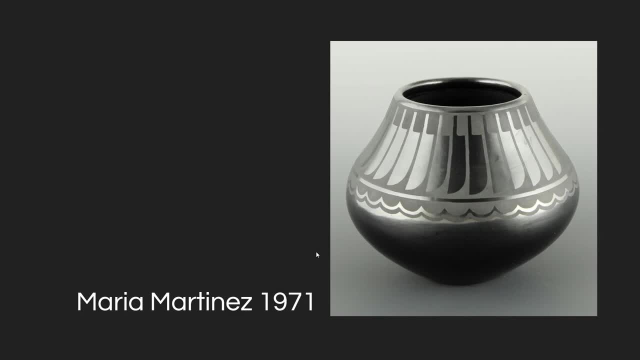 process And then when it comes out it's black. Okay, The clay itself starts off as more of a red clay, So through that whole process it changes it, which is super cool, So definitely check out. I'll have links to either articles or videos for each. 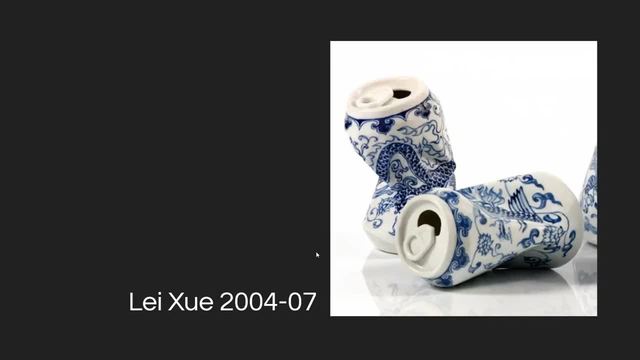 These artists in the description below, if you want to learn a little bit more. The next one is Li Zhu, a Chinese contemporary ceramic artist. They he specifically works with porcelain, and that's why it's super, super white. Okay, Porcelain is a very it's a special type of 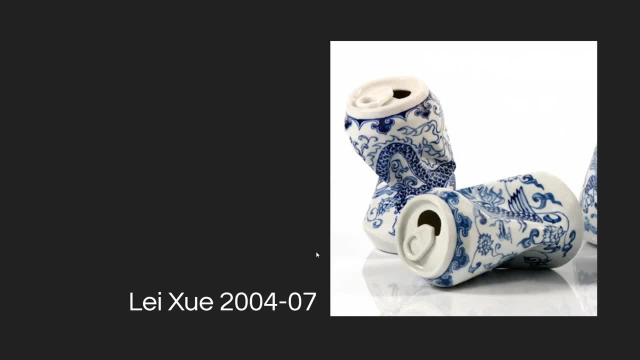 clay. Basically I think of it as something that's much smoother and it also is translucent, which means that a little bit of light kind of shines through the piece. Okay, It doesn't mean I can do it like I see everything, but like it's not completely opaque And also it's fired at a much. 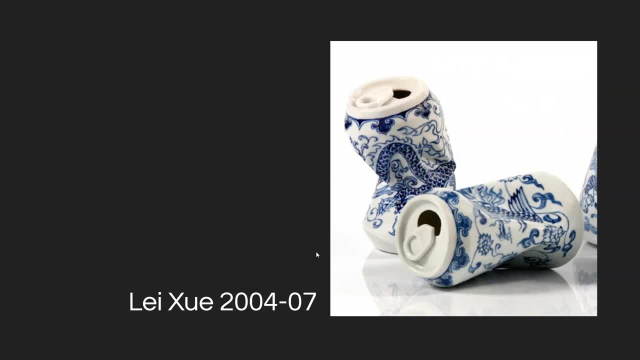 higher temp than a regular stoneware clay is. Anyways, this collection of work that I did- I believe it's called drinking tea, but they, these cans like they look like discarded cans- that are very elaborately painted in that that traditional blue on white kind of style we see. 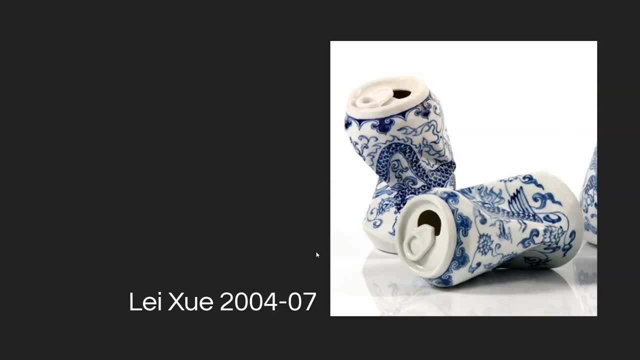 when we think of porcelain plates and things like that, And it's very, very restored to the like that, And each of these are 100% handmade, So he doesn't create a mold and then, uh, slip, cast it. No, no, it's all handmade And he really, and hand painted, for that matter, And he is very 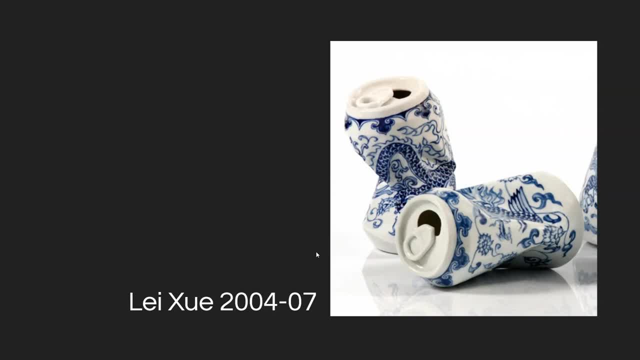 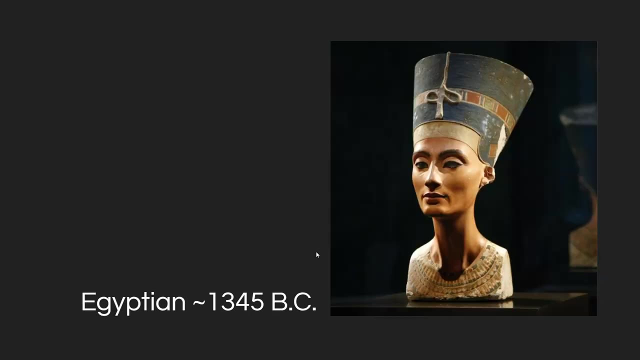 passionate about the hands-on aspect and doing everything start to finish by hand with his work, which is really cool. So definitely another cool artist to check out. Uh, the next two are far more, I guess, old. Okay, Uh, we don't know specifically the artists. We have some ideas for some of them. 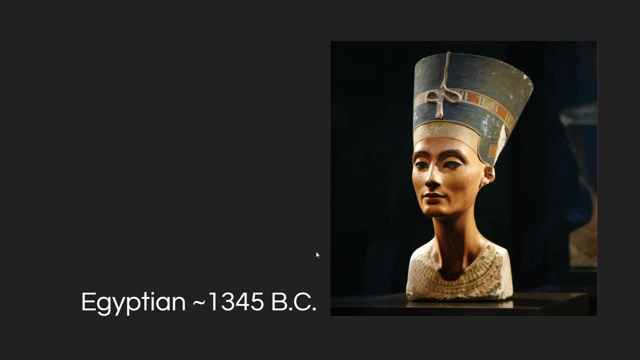 such as this one. This is an Egyptian bust back in like 1345 BC. So if we use some math, 1345 BC that means before, like our zero, on our like timeline that we use. So, whatever year it is, add 1,345 years. So this is, like you know, way over 3000 years old, So it's a very old. 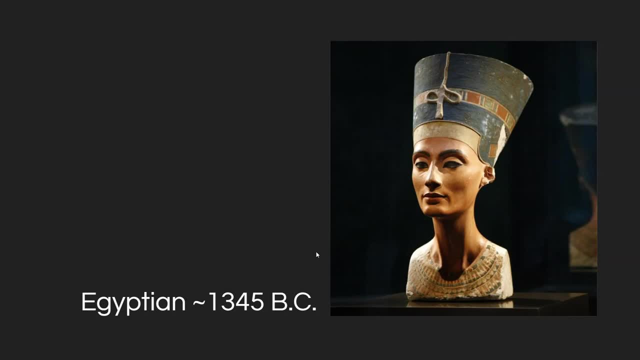 work of art. So, as you can see, ceramic can last a long time. So if you make a bust yourself buried in your backyard, 3000 years from now, someone will find it and be like: Ooh, this is cool, Let's put it. 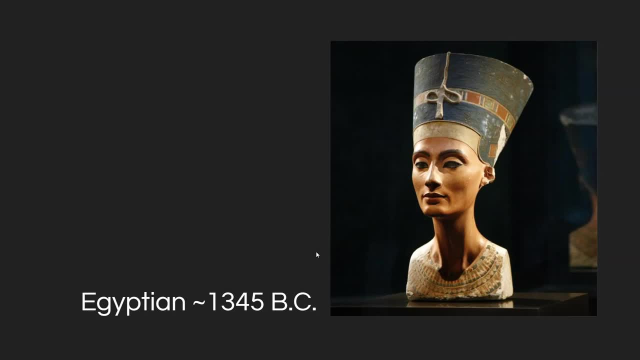 in a museum. Just an idea. Anyways, this is a bust of Nefertiti. She was a queen in Egypt and ended up being a very powerful individual in Egypt, And she and her husband created this- a new religion during the rain and all this crazy stuff. So definitely interesting lady to learn a little. 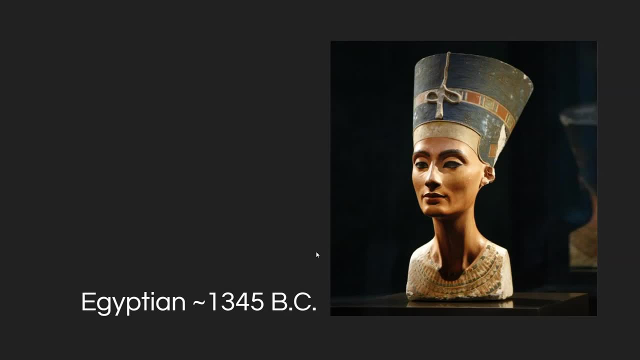 bit more about. So check out that link below. There's a link in the description box below. There's just a short video that talks a little bit about it. But what makes Egyptian work very unique? I like to look at the details and you can really see. you know, kind of like, what they wore. 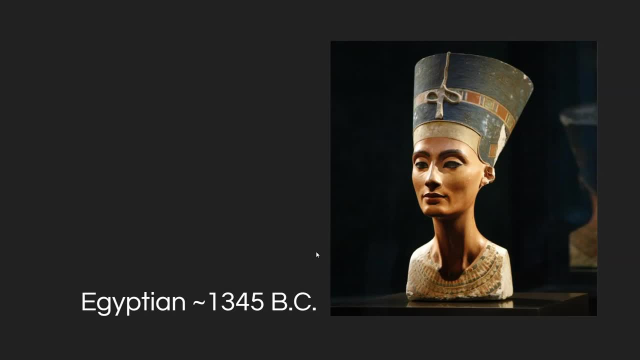 and that kind of stuff. Now the thing is with a bust, you know it's not like a photograph, So we don't know a hundred percent that this is what she looked like. She, you know, Nefertiti means. 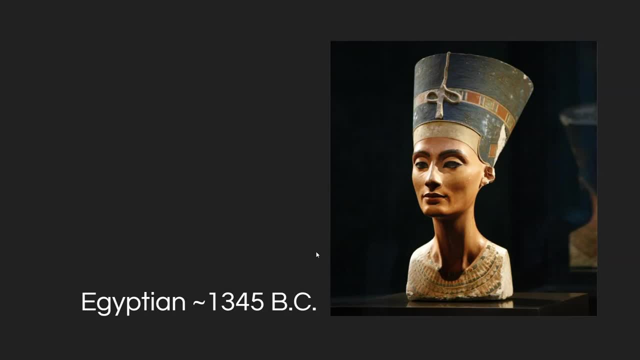 you know, the beautiful one has come, or somewhere close to that translation. I have to Google it again. Anyways, she was known as a very beautiful woman. She was known as a very beautiful woman. She was known as a very beautiful person. So you know, it's either. that's exactly how she looked. 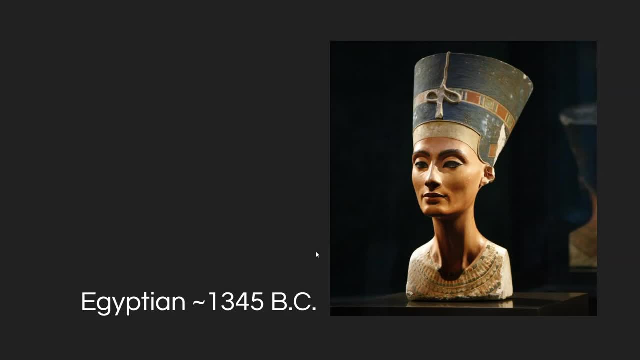 you know cause? you know it looks pretty pretty. Yeah, Yeah, It looks really nice, Or it's. you know how she was portrayed by the artist. I believe it's Thutmose, they believe may have been the one to create this bust. Regardless, in this portrayal she looks very regal, very strong. 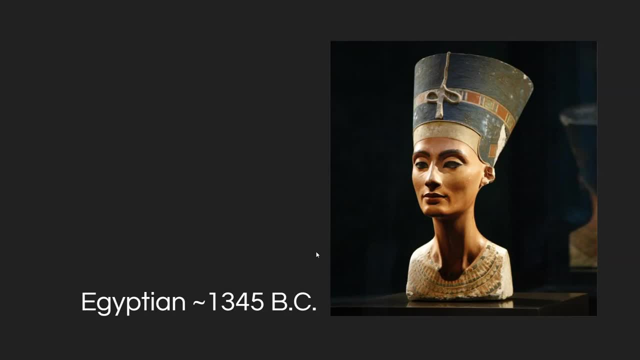 very beautiful And oftentimes she was depicted wearing that sort of Pharaoh, I guess, hat, I guess, like her husband was to sort of like really emphasize the fact that she's a very powerful person. Anyways, Google her a little bit more. Egyptian history is pretty rad, Anyways, last one, 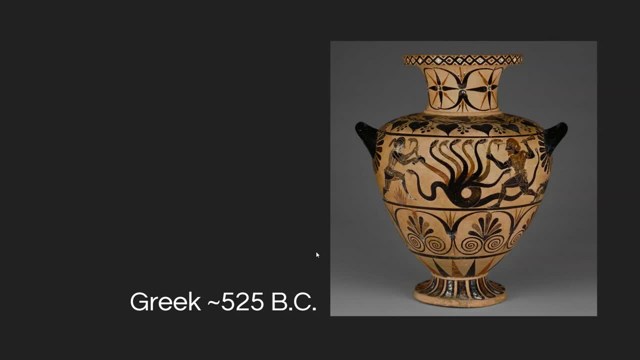 that I want to share with you is a bit of Greek pottery Cause. when I think of pottery and ceramics, I automatically think of Greece. Maybe it's cause I got to go there one time. Anyways, this was created about 521, 25 BC, So not quite as old as Nefertiti, but, you know, just as cool And they. 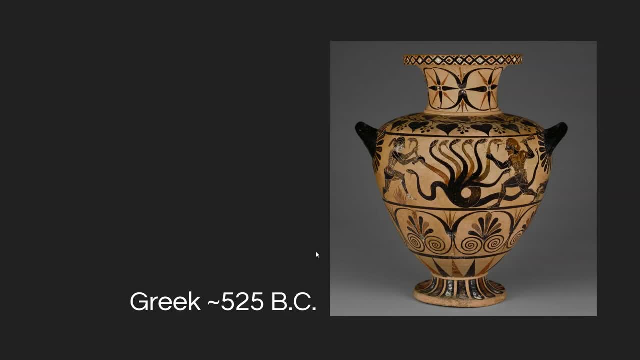 did a lot of experimentation with, like they have this black painting where they go through this process of heating it and getting it, you know, doing all these special things, letting air into the kiln at the right time and all this kind of stuff to oxidize the paint. That's what we get. 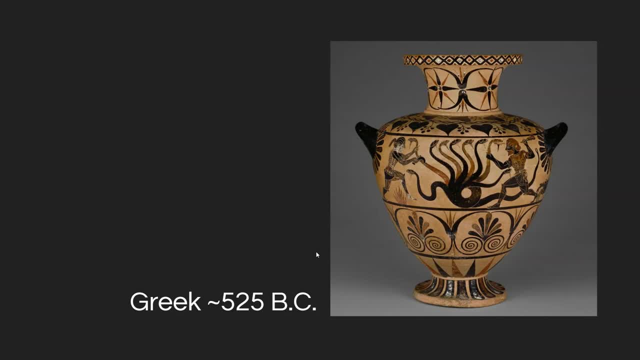 That's how we get the black and the reds showing up just nicely. But a lot of Greek pottery actually depicts, like history and tales of the gods And you know, the demigods, like Hercules, feats of heroism, all that kind of stuff is depicted along. 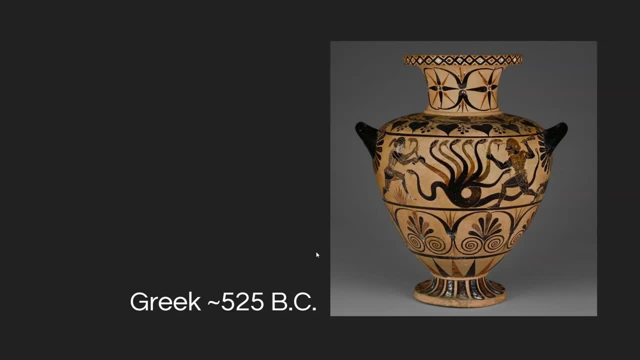 with some you know, traditional motifs in the decorativeness across the lip there and across the base, And these pots were thrown on a wheel, on a wheel. So just like that wheel throwing vid we saw right at the beginning they were created on a wheel. However, when they worked with it, 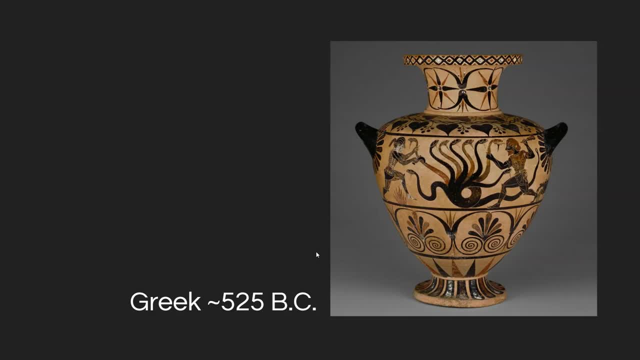 they actually, you know, the potter themselves had to like hand turn the wheel or have an assistant spin it for them. You know, that's a great gift And they make the pot and then they add later the foot, which is what we call that little base, and 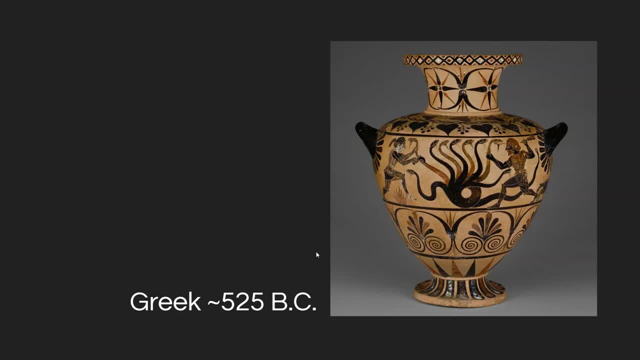 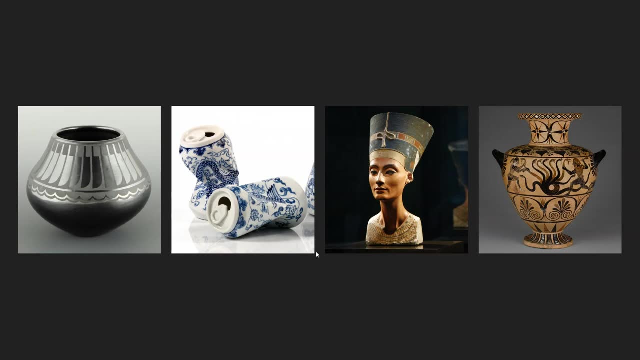 then add the handles and things like that later on. Anyways, one thing I do want you guys to see is like have these all side by side and notice how very different they are. Okay, We have something utilitarian like the black pottery of Maria Martinez and the Greek pot, And then we got the 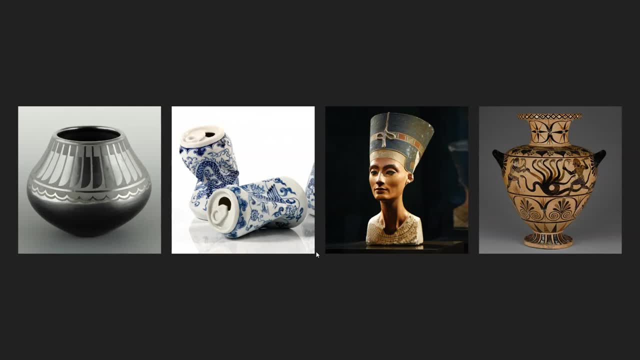 two in the middle which are more sculptural- Okay. And notice how they also look very different from each other. We got one that's very black, Okay, And then we got the porcelain, which is lighter and translucent, And then you got the stone- earthenware in our more ancient 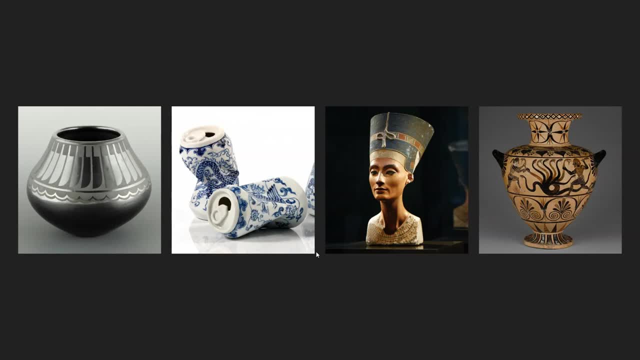 I guess we call it pieces. So there's a wide range for how ceramic can look. There's no specific way because there's so much you can do with clay. Anyways, I hope this is a- you know- helpful little introduction on you know what clay is and some ideas of you know where clay has come.